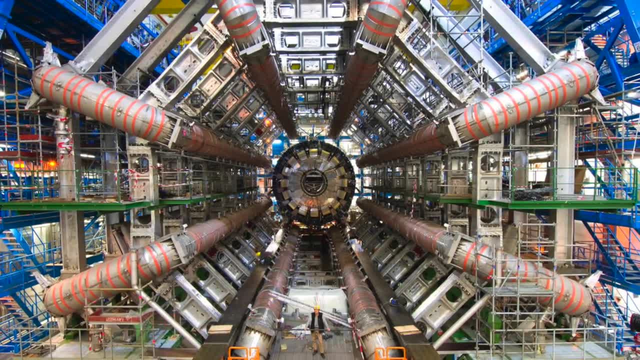 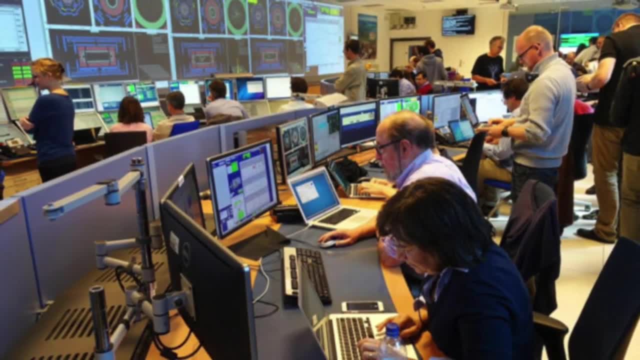 supersymmetric particles could, it's been suggested, be the source of dark matter? The Increased Collision Rate of Super-Symmetric Particles is the lowest of the three, and the most common problem is found in these areas: Precision, energy and the higher collision rate provided by Run 2, as well as new search algorithms. 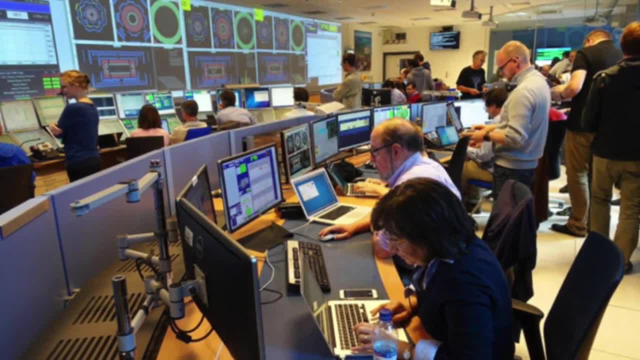 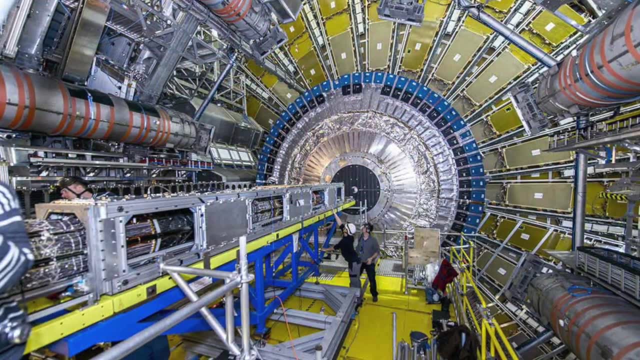 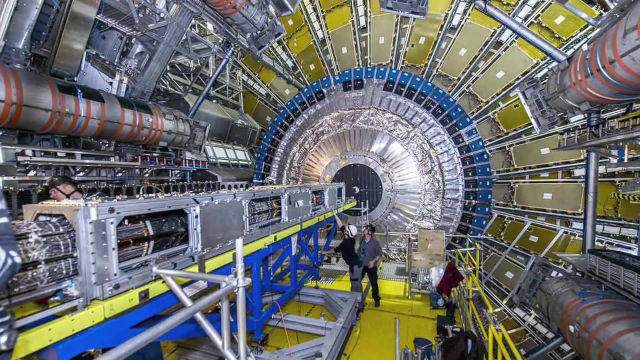 and machine learning techniques have enabled a deeper exploration of a hard-to-reach realm of supersymmetry. The ATLAS team have now presented results from eight separate searches, each looking for evidence of supersymmetric particles in a different way. The combined power and sensitivity. of the various search strategies have proven their relevance to the status quo. The ATLAS team, which has received 18 search reports about the�� and the non-baptist that were done in the past few months, have also conducted experiments to determine if a supersymmetric 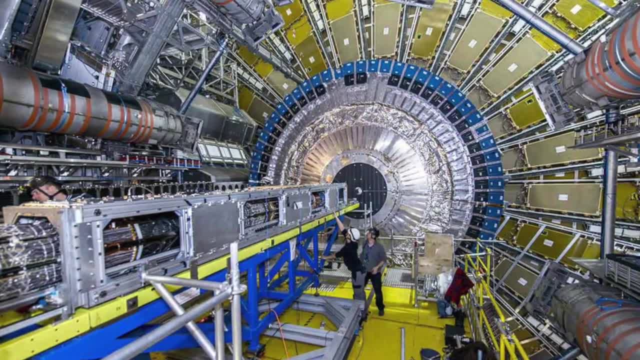 particle is possible or not. At this point, the public has not been able to determine the magnitude of the supersymmetric particles. If a separate sensory probe has been found, they will not be able. has allowed the researchers to test tens of thousands of supersymmetry models. 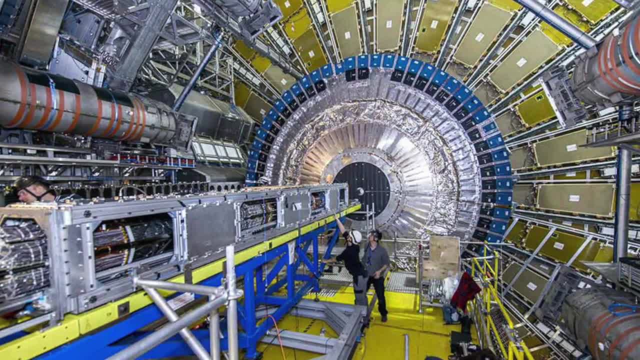 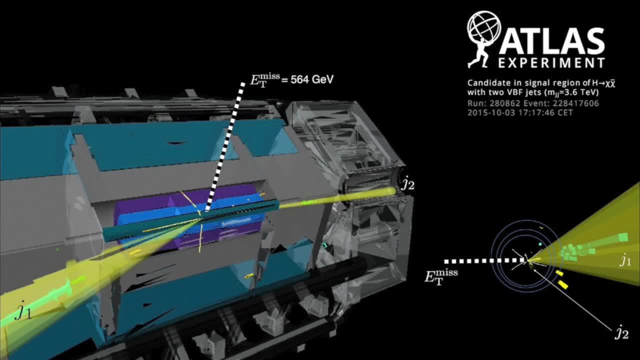 each with different predictions about the masses of supersymmetric particles. The searchers have unprecedented sensitivity and explore a wide range of supersymmetric particle masses. The Atlas team looked for evidence of lab-formed dark matter, In other words, dark matter created transiently during LHC collisions. 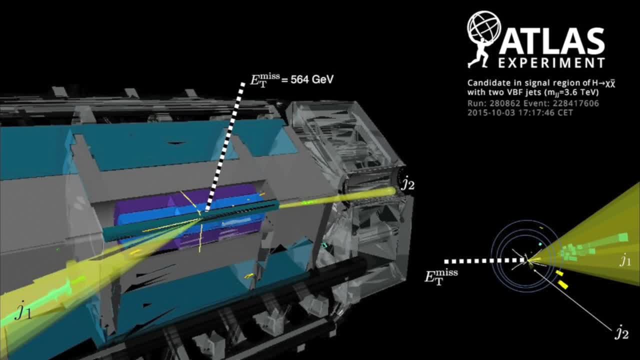 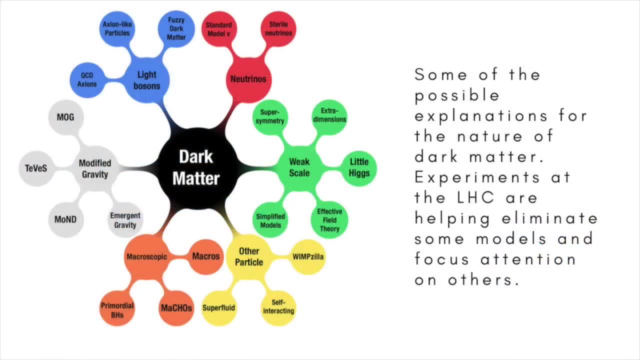 These efforts have proved complimentary to other experiments seeking natural relic dark matter left over from the Big Bang. One of the most significant findings of this combination of searches is that some regions of supersymmetric particle masses that were previously viewed favorably, where the dark matter particle has about half the mass, 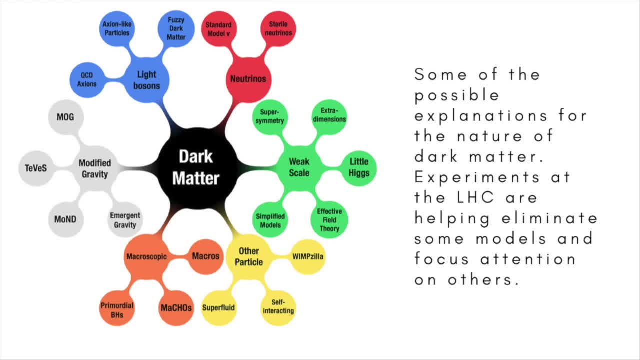 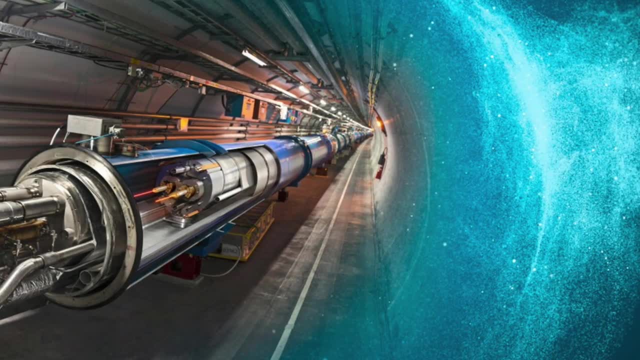 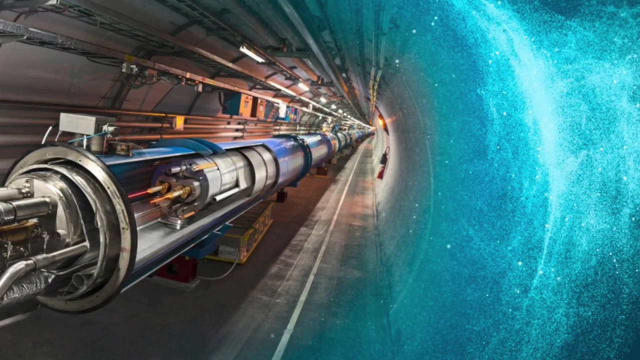 of the Z boson or the Higgs boson have now been almost totally ruled out. Another benefit of such a comprehensive study is an understanding of which supersymmetry models haven't yet been probed. Atlas has presented examples of such surviving models. 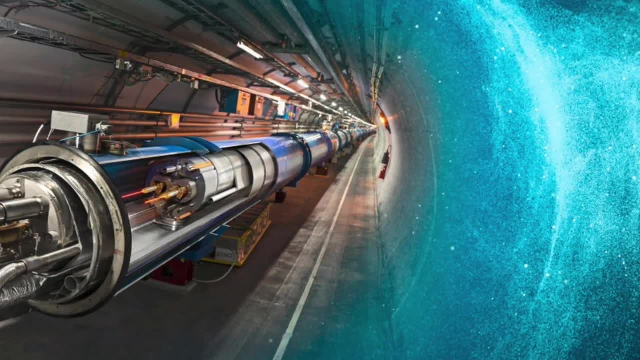 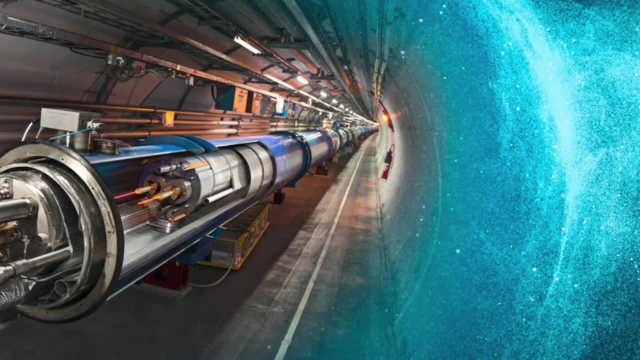 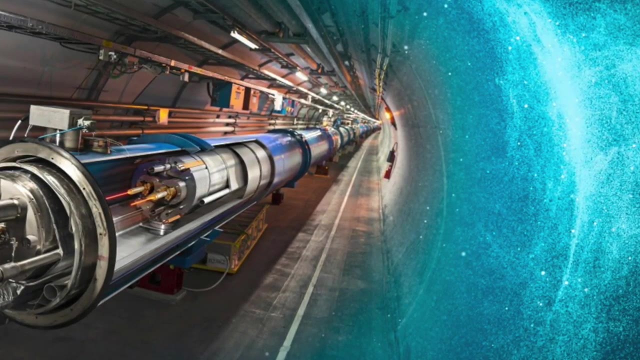 which can be used to optimize future searches. Though possible hiding places for supersymmetric particles are being systematically reduced, many models remain stubbornly elusive. Improving the sensitivity of Atlas searches to these models will require more collision data and further ingenious developments in search strategy.